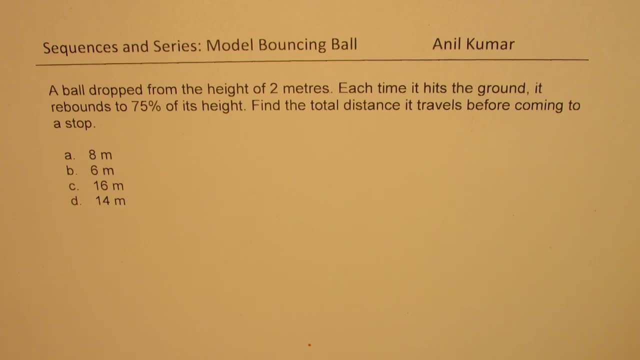 of its height. Find the total distance it travels before coming to stop. Four choices are given to you. Now let's try to understand the situation, and then we are going to answer this. So let's say a ball is dropped like this. Now I'll just stretch it away to show you what is really. 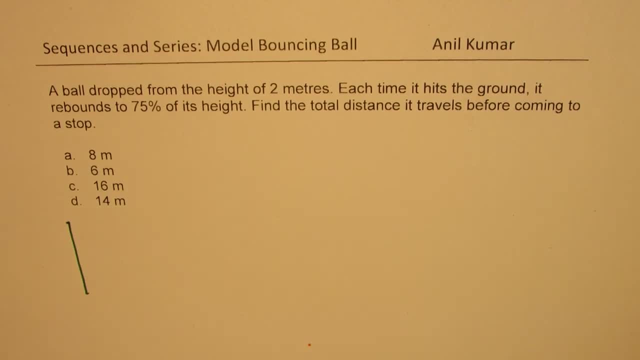 happening, And let's assume that the ground is kind of like this: So when it drops down, it goes up to only 75% of the height, and then again it drops. So like this it goes, and this is how, with time, you will see the height, So it is decreasing. 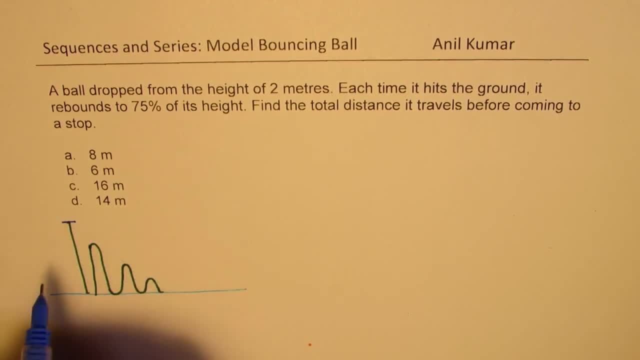 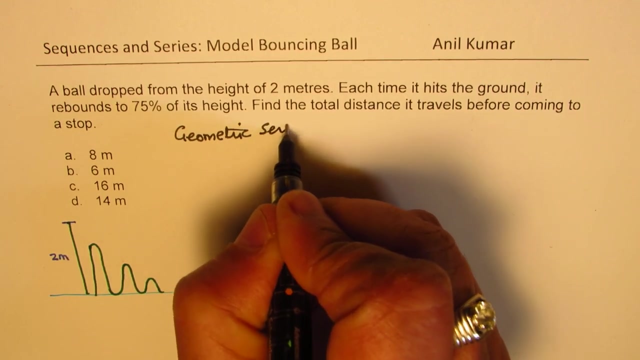 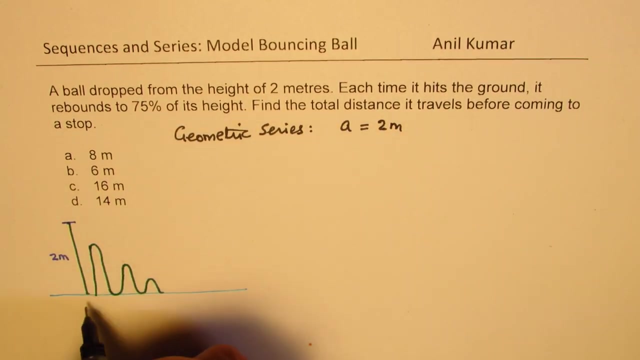 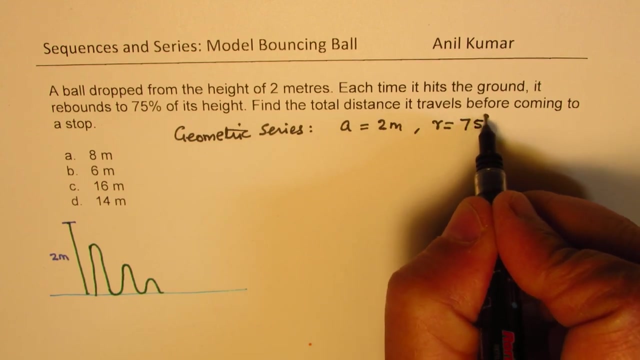 by 75%. We are given that initially the height is two meters, We need to find the total distance. So clearly this is a geometric series right, where the initial value A is two meters for us, and when it rebounds, the factor by which is being multiplied is 75%. 75% means 0.75.. 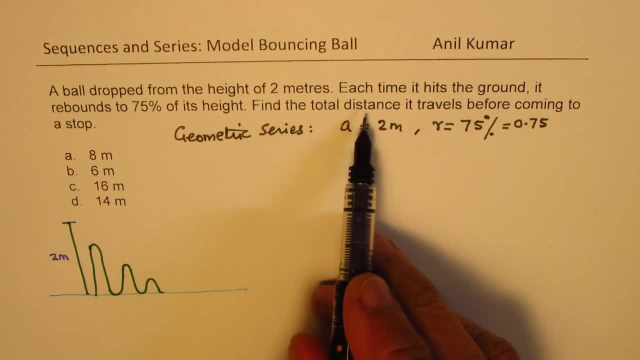 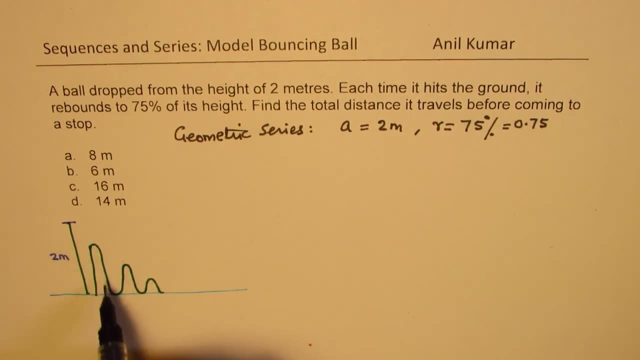 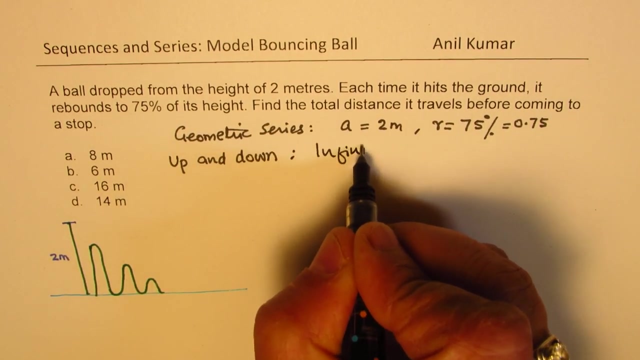 Correct. We need to find distance. so, as you can see here, distance is coming down as well as going up, so so the total distance is both up and and down distance. this is important to understand, correct? so let us assume that this continues forever. so it is kind of an infinite series. so sum of infinite. 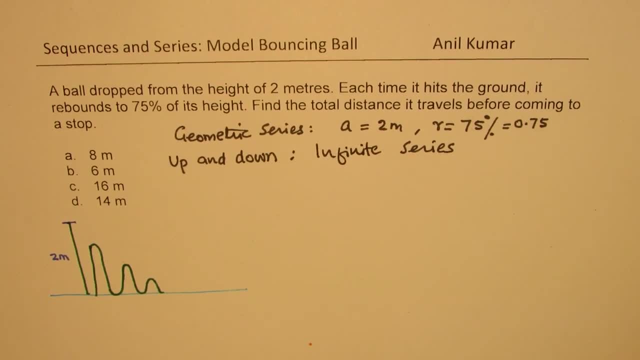 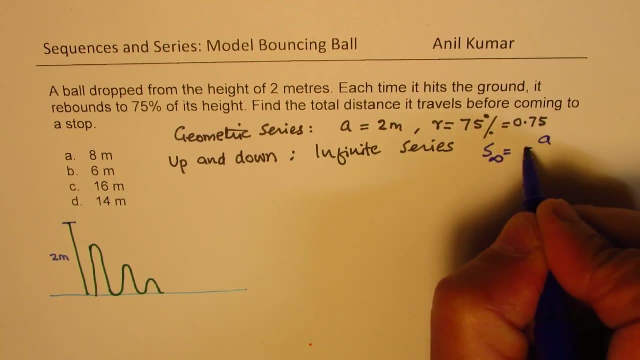 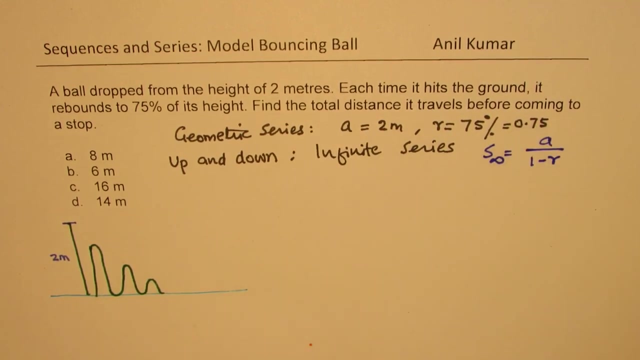 series provides us the solution clear and therefore we can use the formula which is: sum of infinite series is the initial value over one minus R. now the value of R is zero point seven five. so it converges right. So it is converging series If r is less than 1, right. 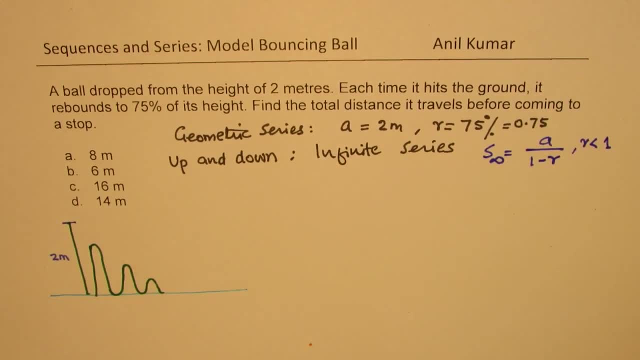 So if r is less than 1, it can be applied. Perfect. So let's apply this formula and find the sum. So sum of infinite series will give us a values 2 over 1 minus 0.75.. 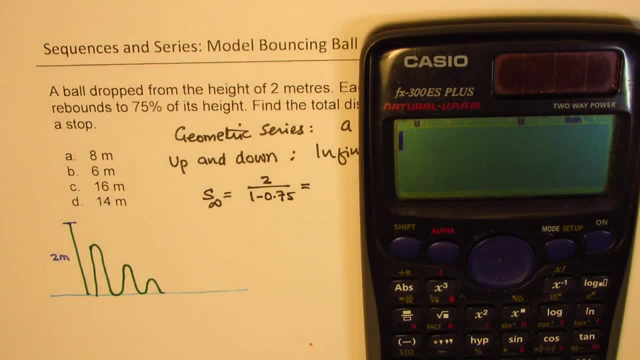 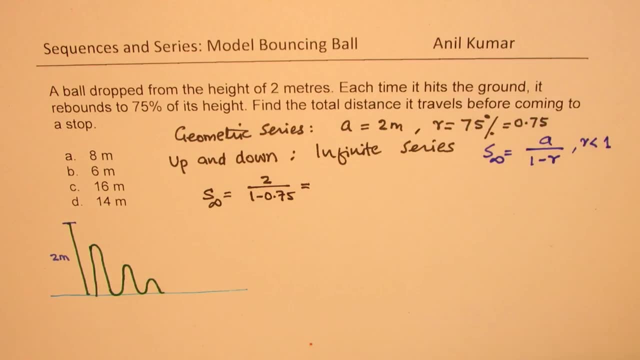 And that is equal to what? 2 divided by, within brackets, 1 minus 0.75, which is equal to 8.. Well, 8 is one of the options. However, do you think it is the right answer? 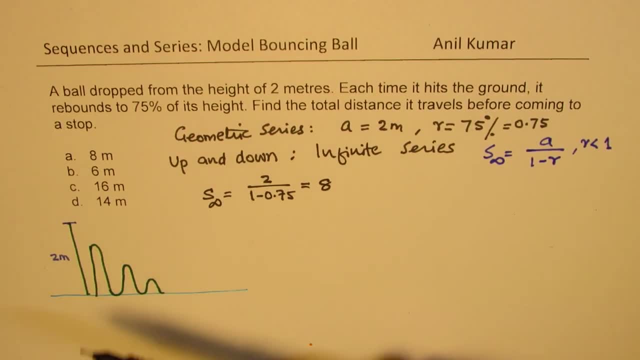 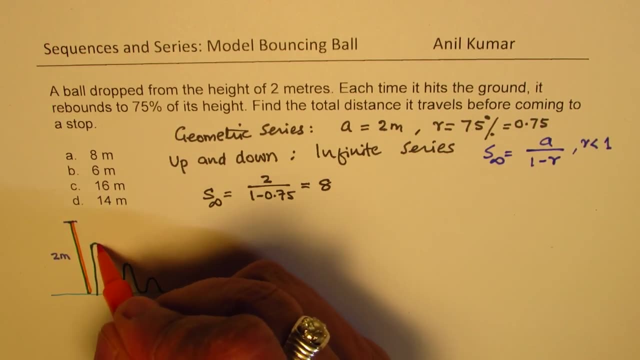 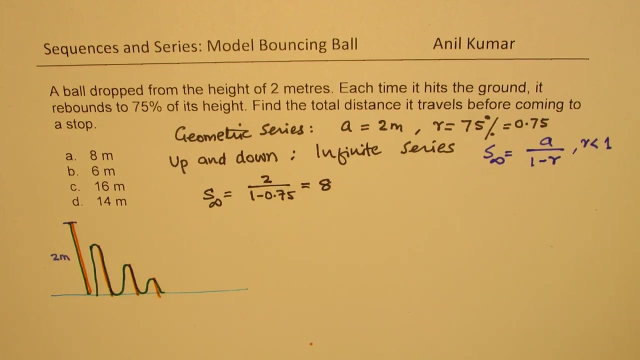 Well, it is not right answer because this only gives you one way, right? So it is telling you that it was dropped. And the second time again, it is only telling you sum of these distances coming downwards, right? So how much is the total distance? 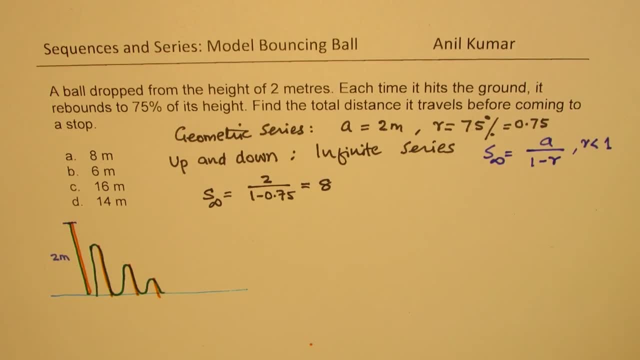 Well, the total distance is that it is also bouncing back. So we have to add those distances which are going upwards also. Do you see that part? So total distance has to be taken. So except for these, all other distances are repeated. 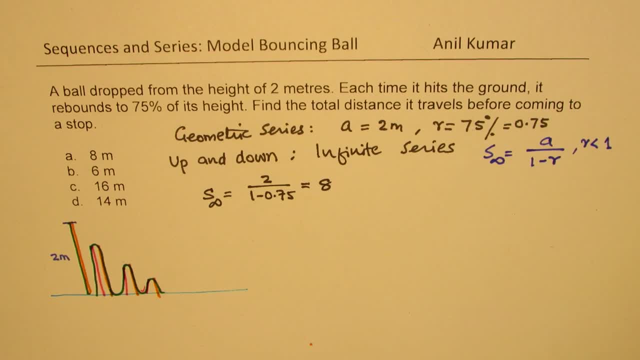 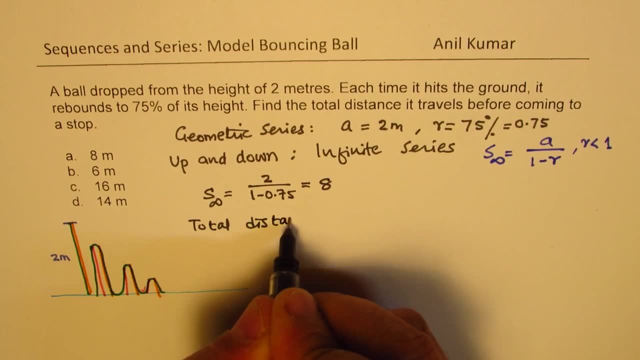 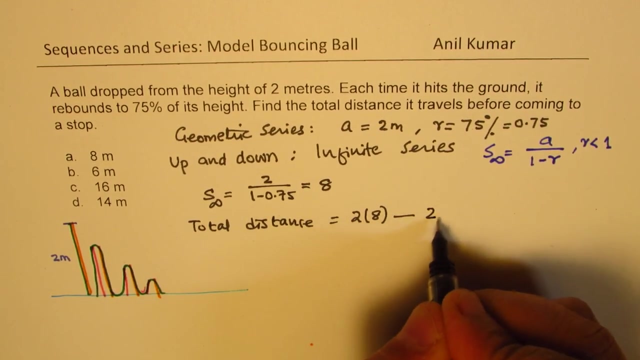 Correct. This is only once, So how do we find The total distance covered? So total distance will be 2 times 8 minus 2 meters. Since it is not going up 2 meters, right, It only falls 2 meters. 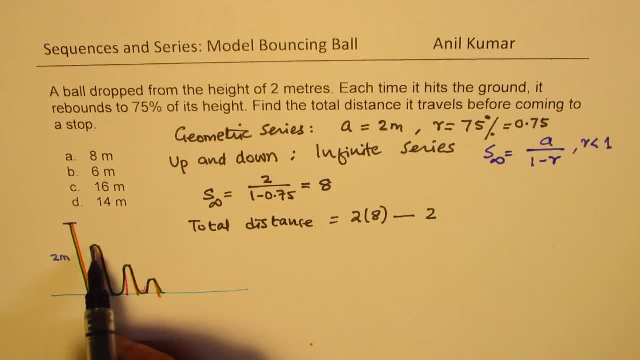 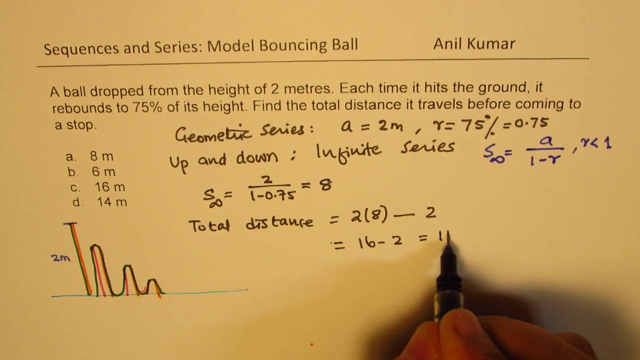 All other distances have been covered twice, right? It goes up and falls the same distance, So twice it is covering from here to there, right? So 2.. 2 times this minus 2 should be the correct answer. We have 16 minus 2, which is 14 meters, correct? 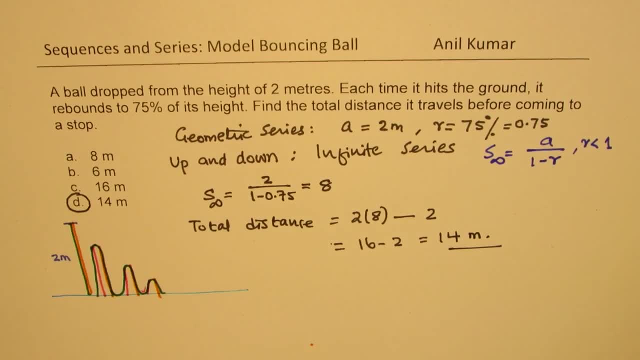 So 14 meters is the right option, which is option D. So this is very important as most of the numbers here may relate some way or the other your values in the solution. However, you should be very clear that when you have a question like this,